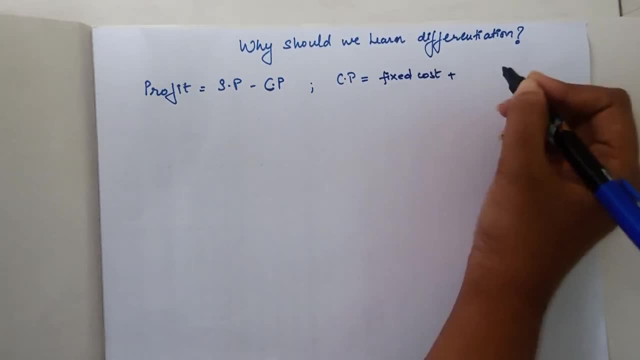 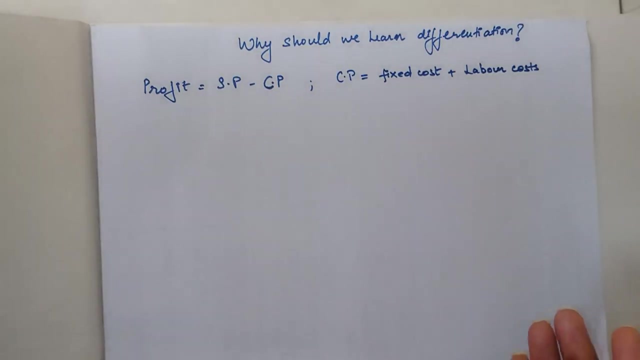 So fixed cost and let us say the variable cost in our venture is nothing but the labor costs. Just to clear: fixed costs are those costs which will be incurred every month. So basically you can include Cost such as rent, electricity in fixed costs. 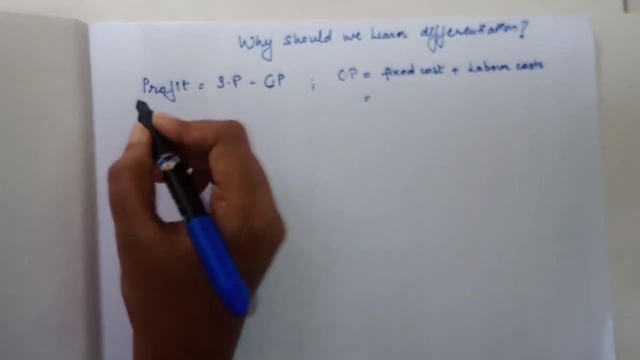 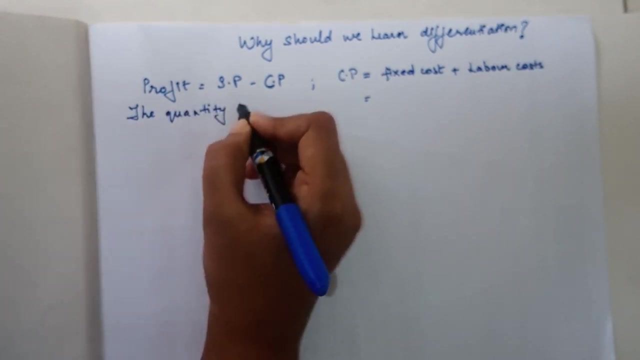 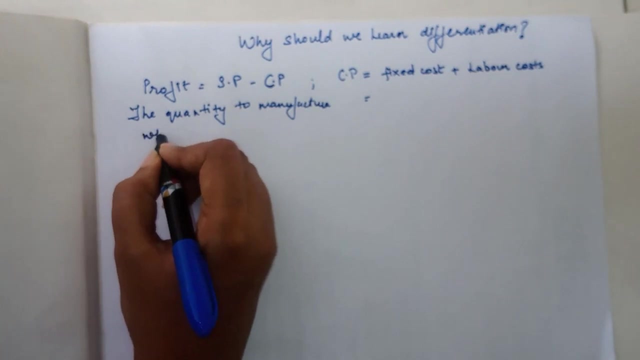 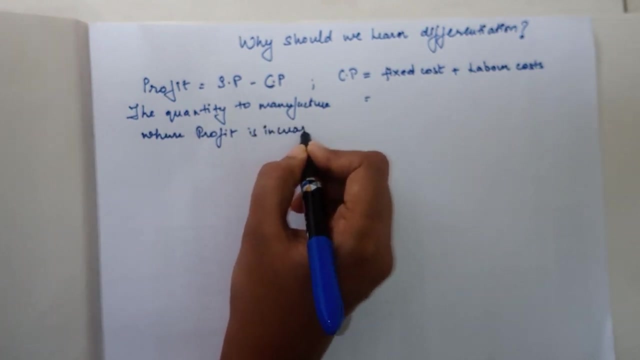 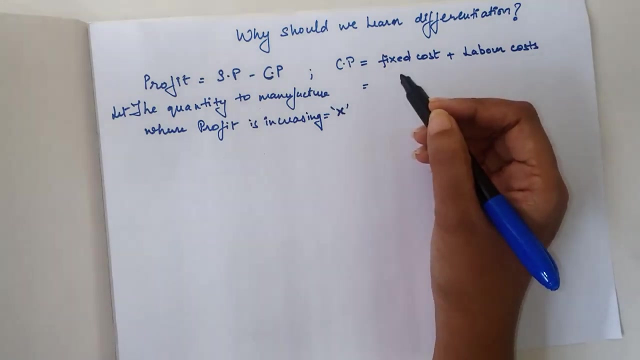 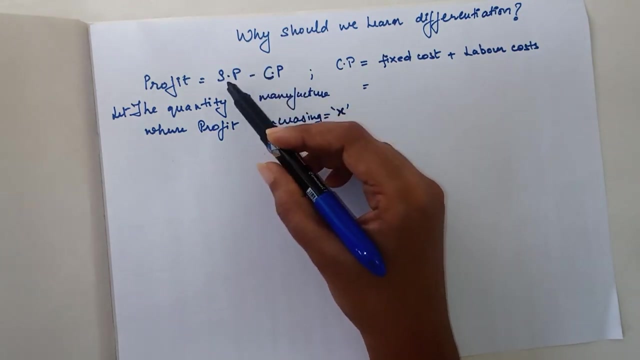 And since students I want to figure out the profit. I need to figure out the quantity to manufacture where profit is increasing. Correct, Now let us name that quantity as X. So we will try. So now we will put all the values of cost price as well as selling price in terms of X. 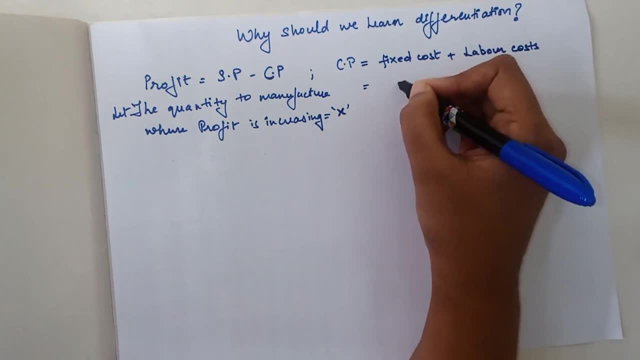 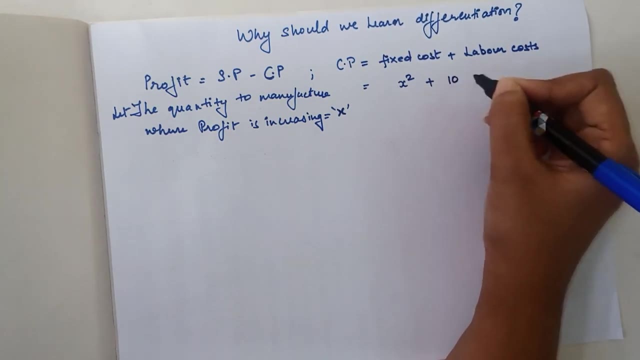 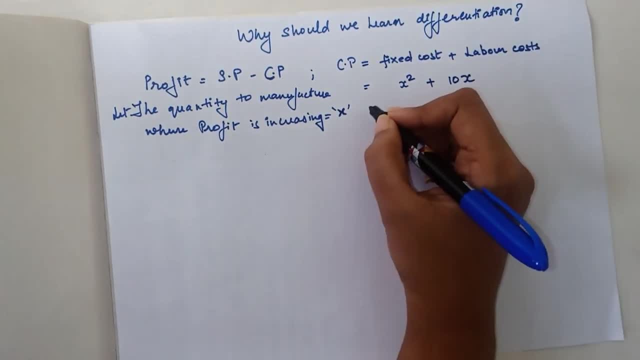 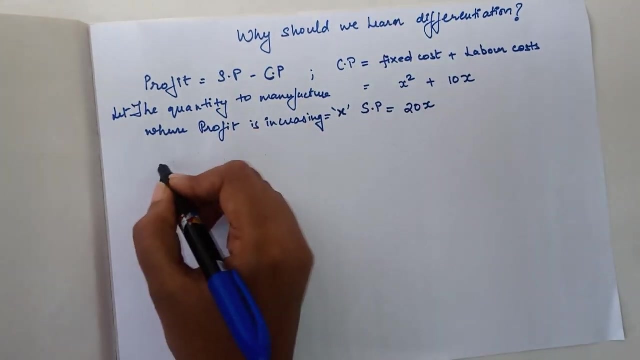 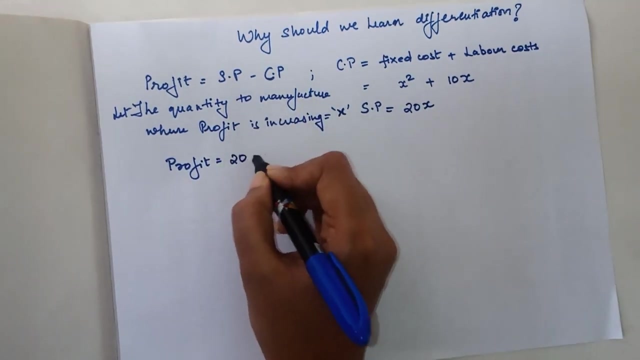 It would be 10X And we plan to sell each of our pen at rupees 20.. So the selling price for X pens would be 20X. So from here I can say that profit is equals to SP, which is 20X, minus cost price, which is X square. 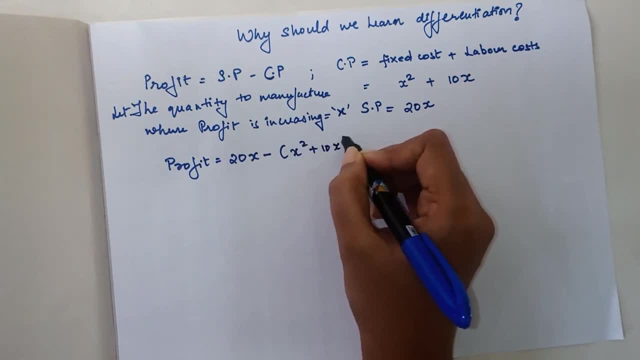 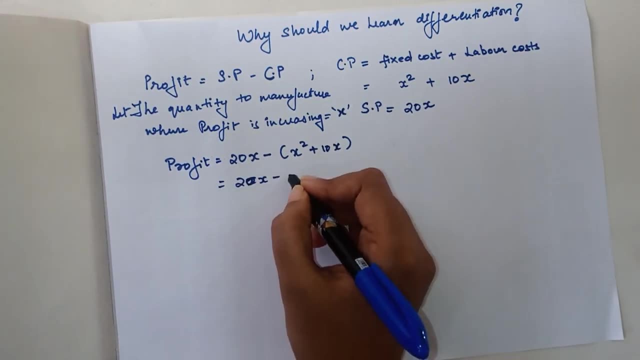 So from here I can say that profit is equals to SP, which is 20X minus cost price, which is X square plus 10x. opening the brackets, we get 20x minus x square minus 10x, which is equals to 10x minus x square. since I need to find out the value of x for 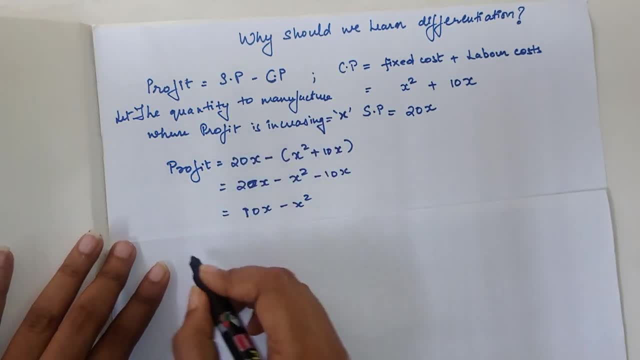 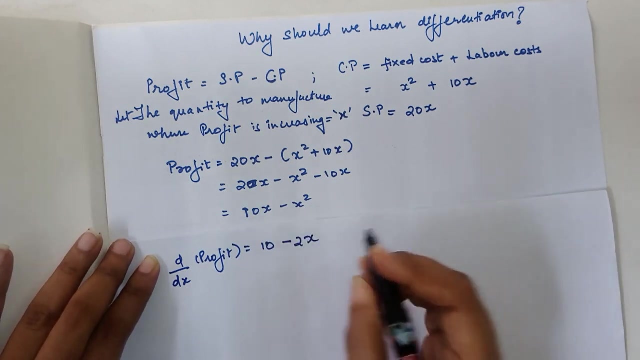 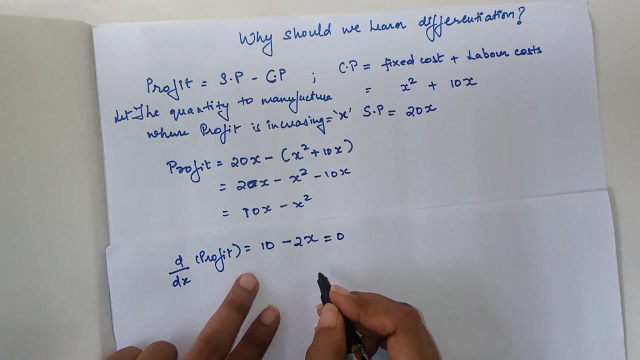 which my profit is increasing. I am just simply going to differentiate profit with respect to x. so differentiation of 10x gives me 10, and differentiation of minus x square gives me minus 2x. and since I need the profit to be increasing, I am just going to equate it to 0. so from here I can say my value of x equals.